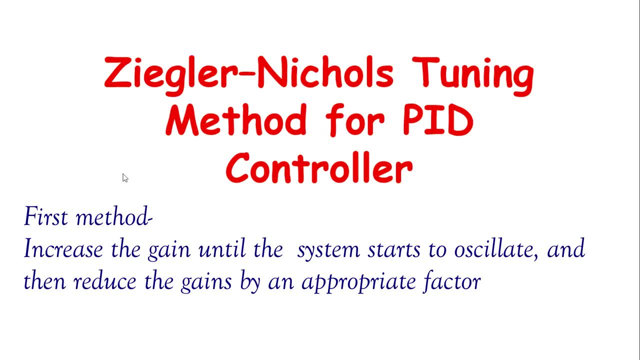 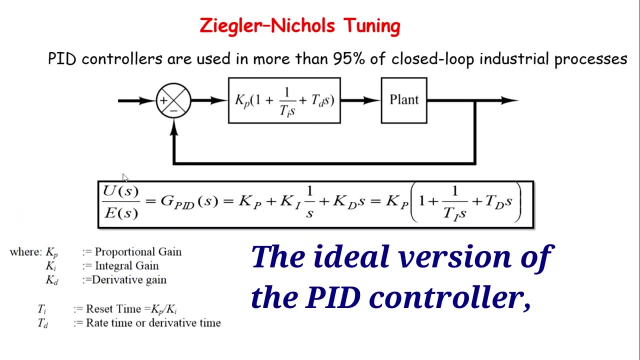 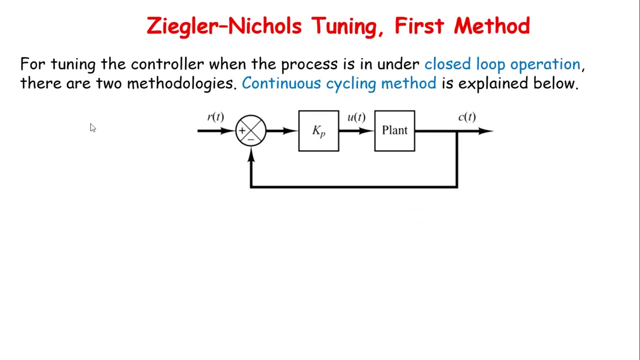 increase the gain until the system starts to oscillate and then reduce the gain by an appropriate factor. Another method is to measure some features of the open-loop response and to determine the controller parameters based on these features. Let us start with the first method of Ziegler-Nichols tuning, based on direct adjustment of controller. 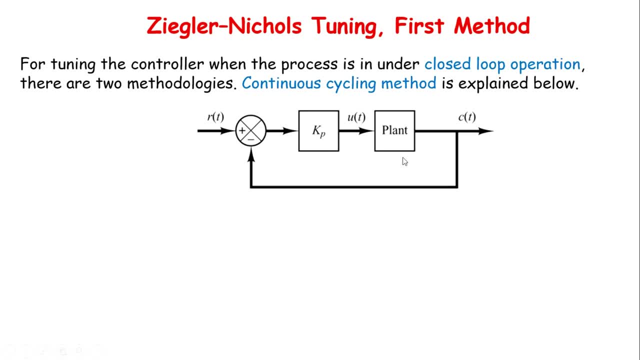 parameters, A controller is connected to the process. Integral and derivative gain are set to zero and proportional gain is increased. until the system starts to oscillate The critical value of proportional gain, the position is set to zero. This is not necessary here. 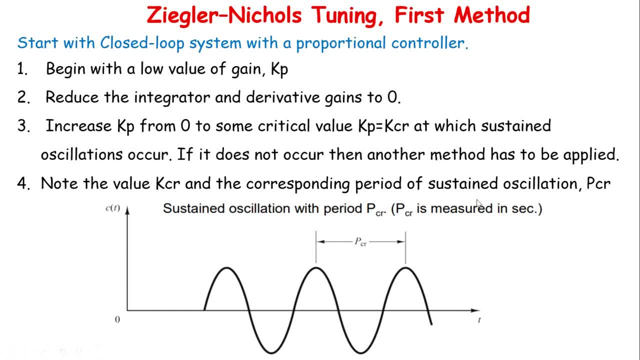 The value of the proportional gain is equal to the swing of force of the controller. Thus, the control parameters are set to zero. The controller diameter is also set to zero. The, that is, kcr, is observed together with the period of oscillation, that is tc, the controller parameter. 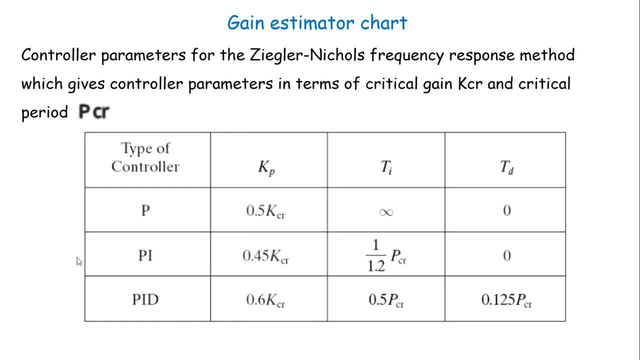 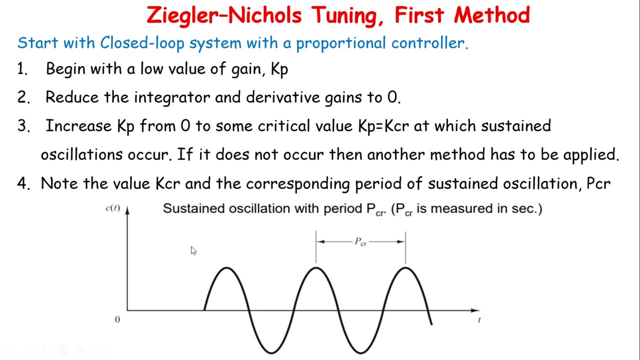 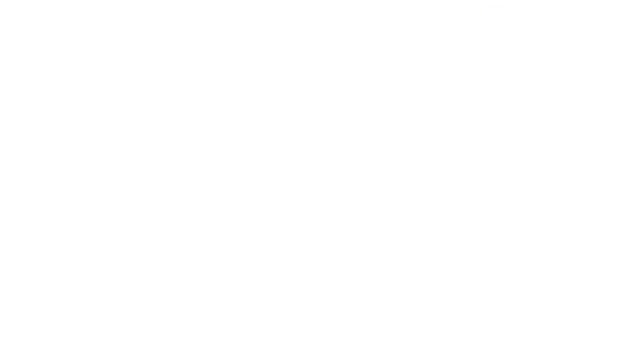 are then given by table. the values in the table were obtained based on many simulations and experiments on process that are normally encountered in process industry. there are many variations of the methods which are widely used in industry. let us see the procedure step by step in brief. first step is first note whether the required proportional controller gain is. 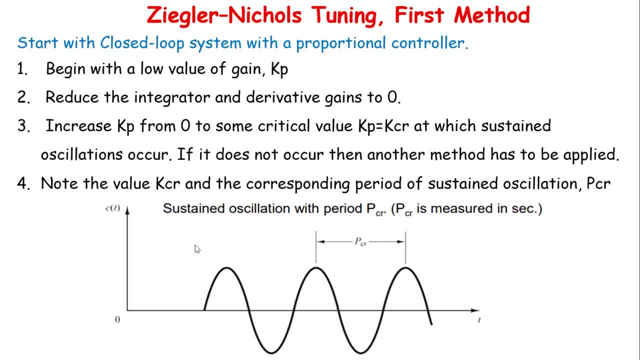 positive or negative. to do so, step the input u up a little under manual control to see if the resulting steady state value of the process output has also moved up. if so, then steady state process gain is positive and require proportional control. gain k has to be positive as well. turns the controller to proportional mode only, that is, turn both. 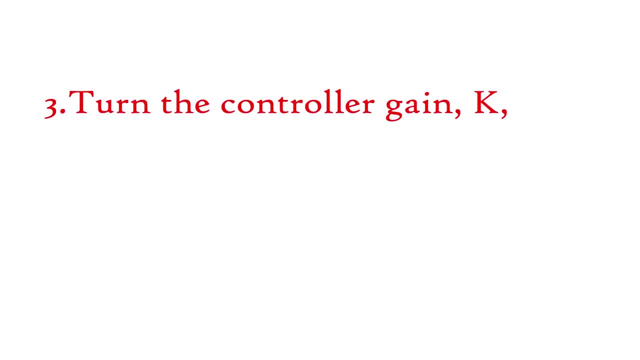 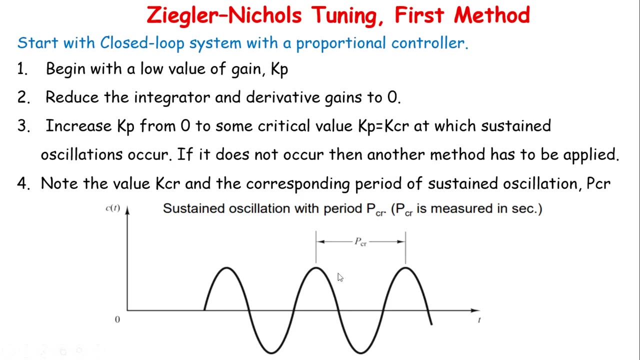 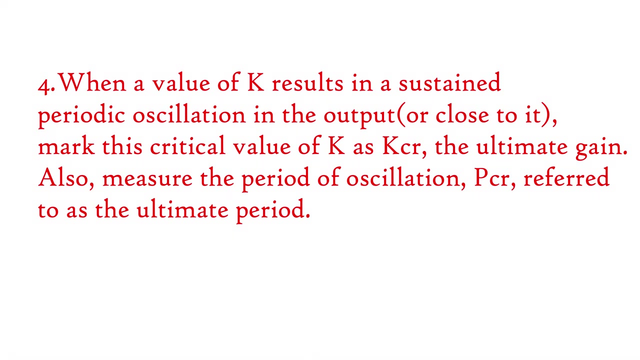 integral and derivative mode off. turn the controller, gain k up slowly and observe the output response. note that this requires changing k in step increments and waiting a steady state in the output before another change in k is implemented. First step is when a value of k results in a sustained periodic oscillation in the output. 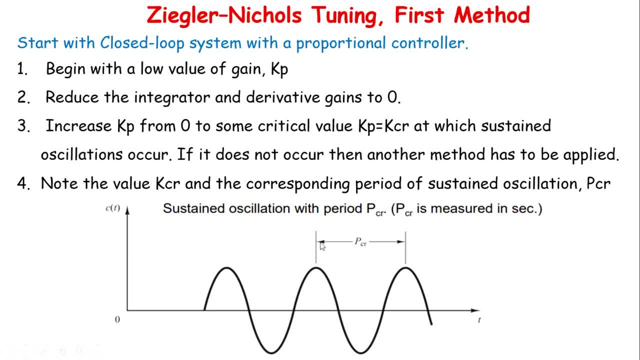 mark this critical value of k as k critical, that is, ultimate gain. Also measure the period of oscillation, that is, pcr referred to as a ultimate period. This is the procedure by which we can do the PID tuning. Let us see another method: Zillow-Nikolaus tuning, based on 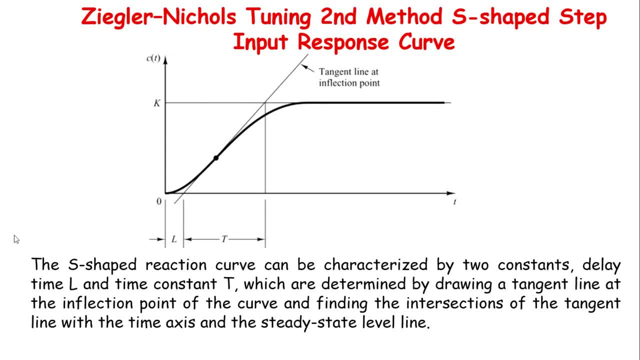 s-shaped step input response curve. This method is based on determination of the open loop step response of the process, as shown in figure. The step response is measured by applying a step input to the PID tuning. This method is based on determination of the open loop step response of the process, as shown in figure. The step response is measured by applying a step input. 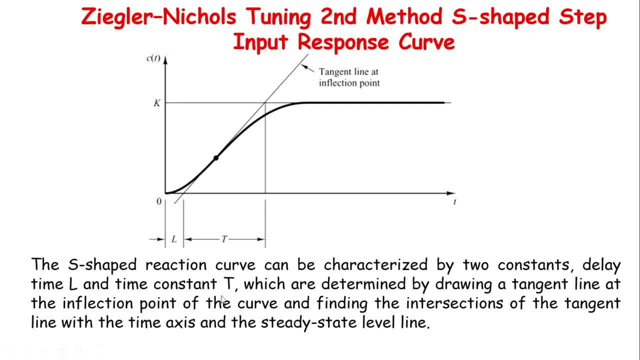 The step response is measured by applying a step input to the process and recording the response. The response is scaled to correspond to a unit step input and characterized by parameters delay time l and time constant t, which are the intercepts of the steepest tangent. 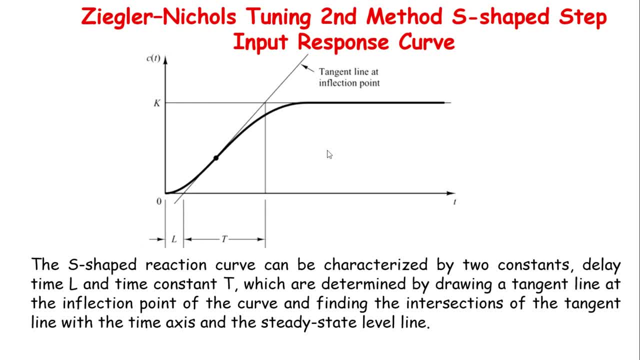 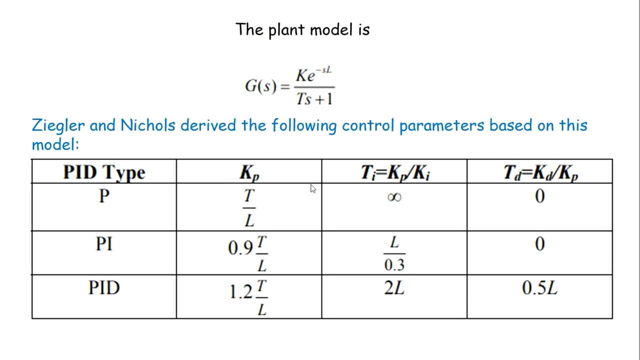 of the step response with the coordinate axis. The parameter t is an approximation of the time delay of the system. Notice that it is not necessary to wait until steady state to find the parameters. It suffices to wait until the response has had an inflection point. The controller parameters are given in a table. 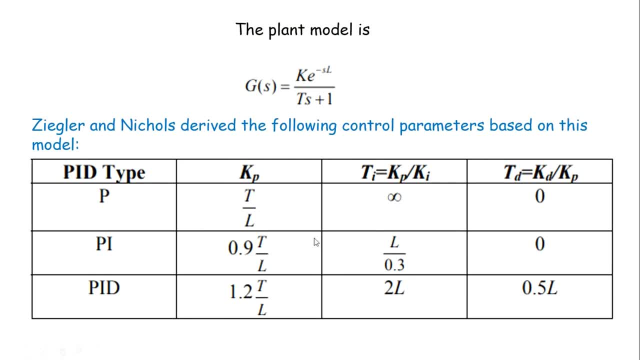 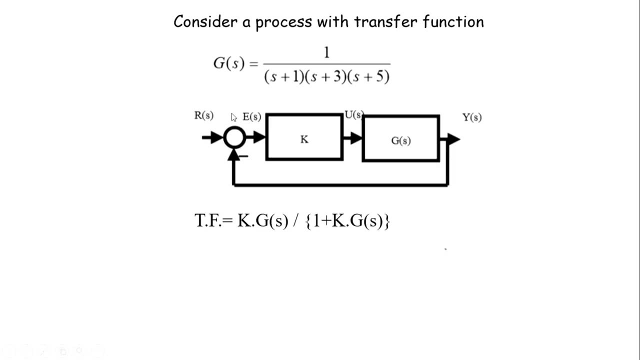 The parameters were obtained by extensive simulation of ranges of representative process, when numerical, based on the PID tuning, Considering the closed loop system we are going to tune, along with amazed, or to find out the value of kp, ki and kd. разб usa observando el sistema de cerros lackados. 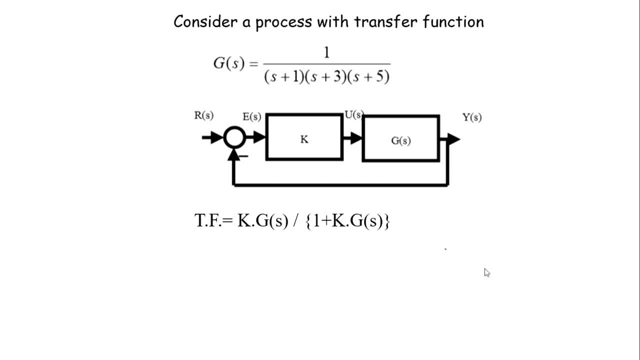 and the transfer function for this system is the following: This is a Shepherd filter grandchildren checkbox. set it in use. do theï ultuitep Call interface checkbox. set it in use. do the✩ Verify. setl sentir briefcase: Rosen and t bananas. We have to find out. 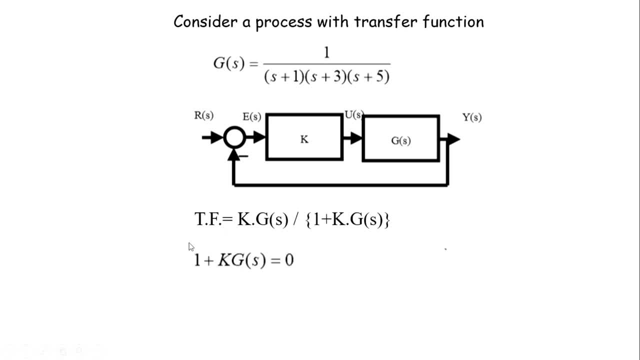 the characteristic equation. so at the denominator. if you solve it, I get the characteristic equation equal to sqion Cornus-집 33 s square sq fingers plus Sq, square sq, ه plus sq. Now we have to determine the area of q. to determine the area of q水ations, we can see aluminium's value of despothem. 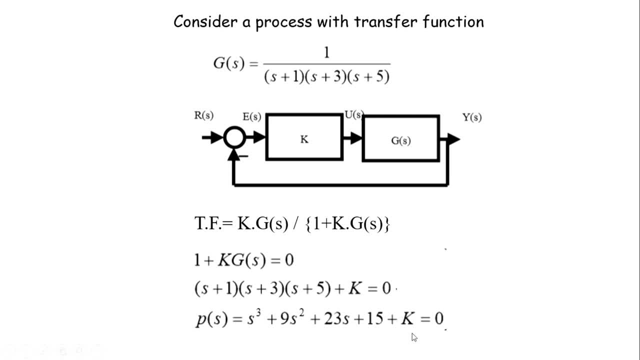 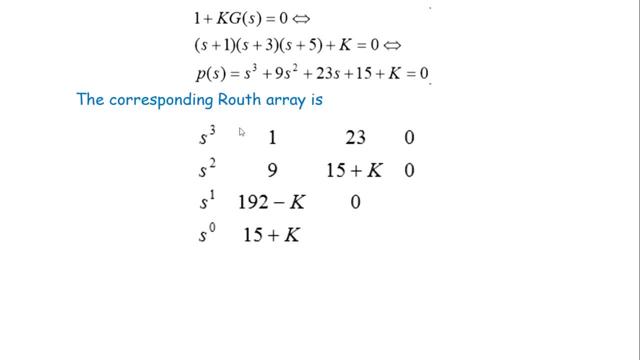 to determine the value of k. i am going to use the root service criteria. it is the root array and that you have to put the all coefficients in respective place to find out the value of k. or how to find out the value of k, please refer my other videos. 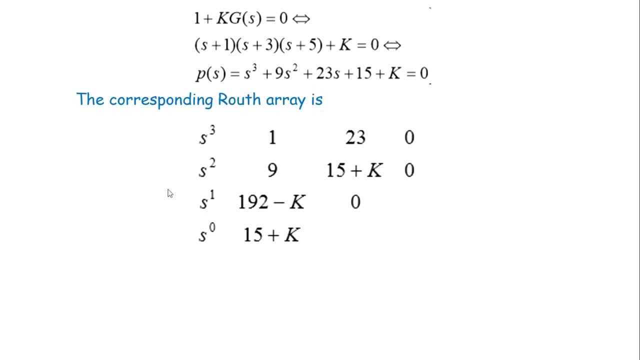 based on the service criteria. right now, here i am directly putting the value of k from my use cases. i am going to see that. let me back to the understanding of the root array. now, from the roots array, from row number S- zero. if you see here, 15 plus k is greater than zero. in that i get the value of k is greater than minus fifty, remember. 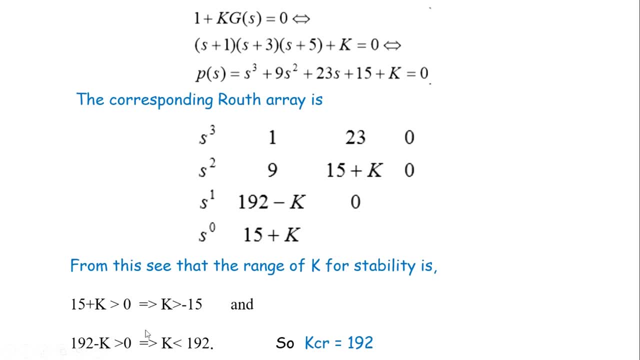 that, as we discussed earlier, we need the gain margin positive. so if you go to the row number value of k, which is less than 192, means here we are having the positive gain. so the well critical value of the gain is 192. now, by considering the row number, 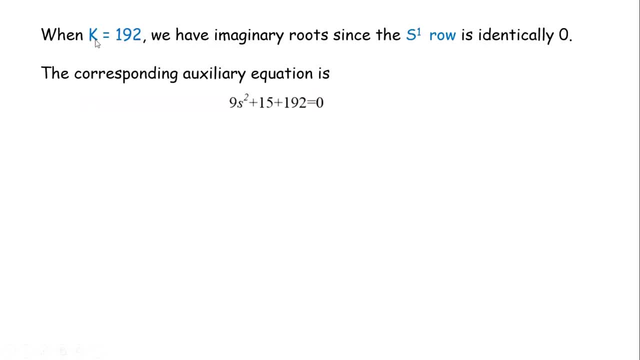 used to the auxiliary equations. we get 9s square plus 15 plus 192. here i have kept the value of k is equal to 192. now, by considering this characteristic equation, if you find the roots, i get the roots: is equal to s, is equal to plus minus j, 4.8. the roots of this equation. this is: 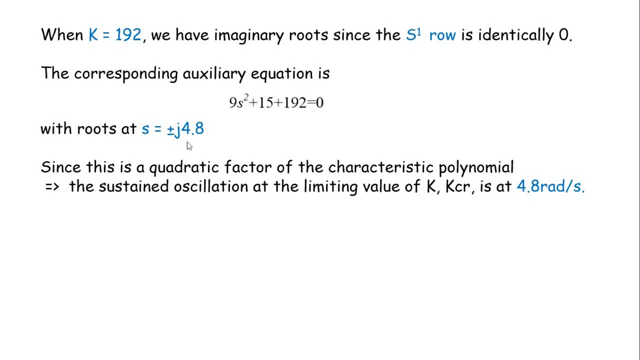 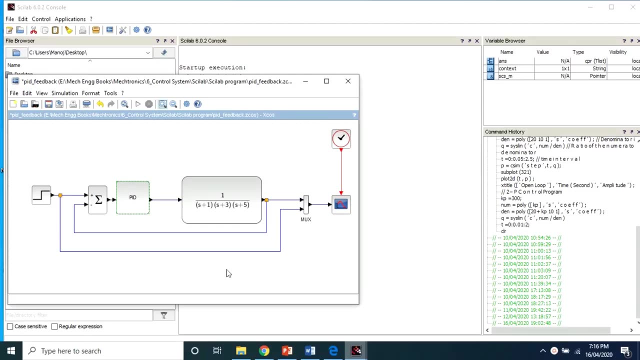 the quadratic factor of the characteristic polynomial. the sustained oscillation at the limiting value of kcr is at 4.8 radian per second. to find out the value of pcr, that is the ultimate period we have to put. the proportional gain is equal to 192. now, this is the transfer function. here i am going to 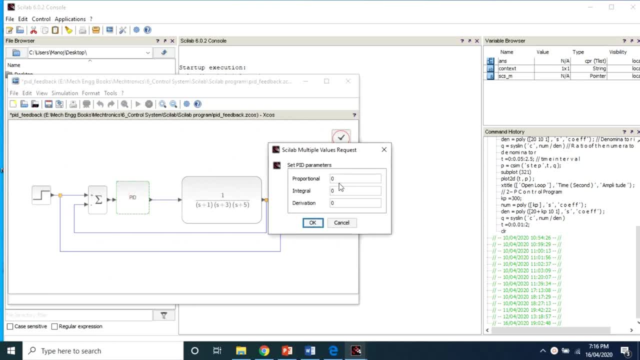 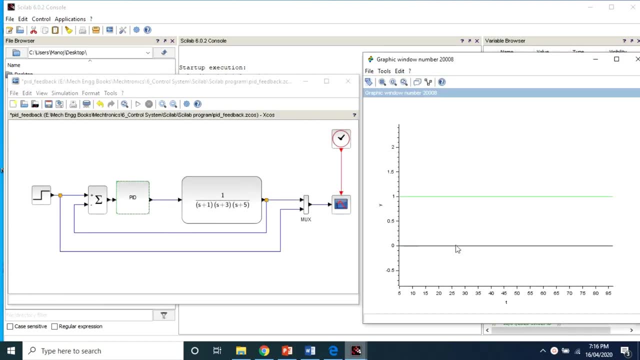 substitute. the value of p is equal to 192. now, first of all, see the response by considering the all constants is equal to zero, see the response curve. you get the horizontal line. now i am going to change. the proportional gain is equal to 192 and see the change into the response curve. 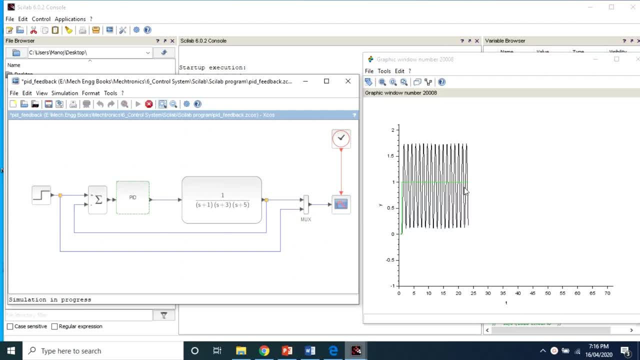 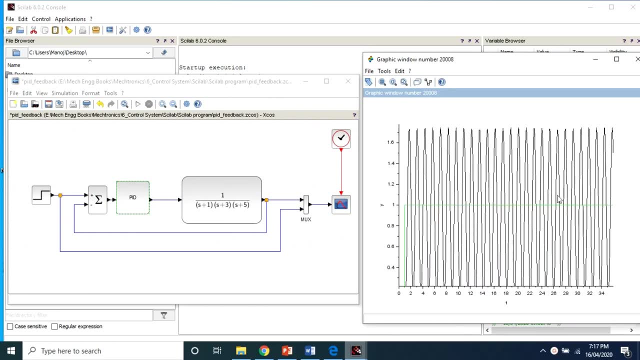 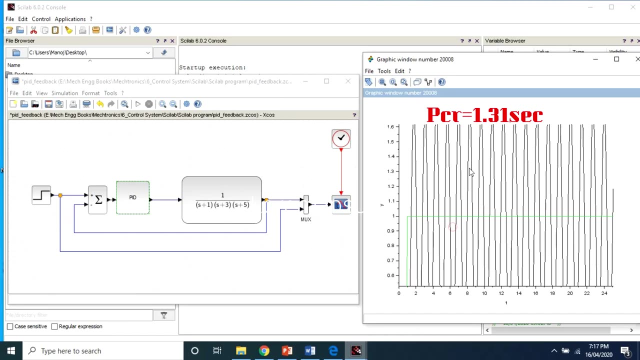 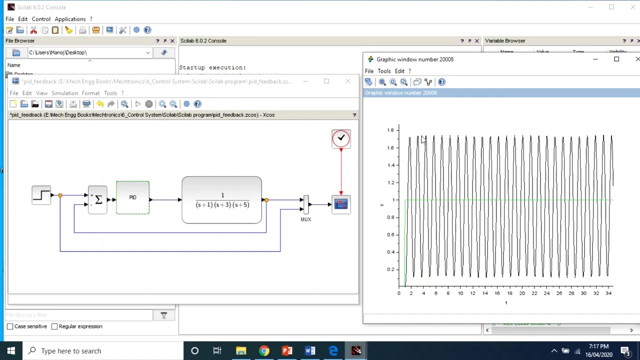 here you get the continuous oscillation, the time between two peaks. okay, this is your ultimate period denoted by pcr, approximately the time between these two peaks is 131 seconds. okay, so by considering this, pcr and kcr, we are going to find out the value of ti and td. we know the 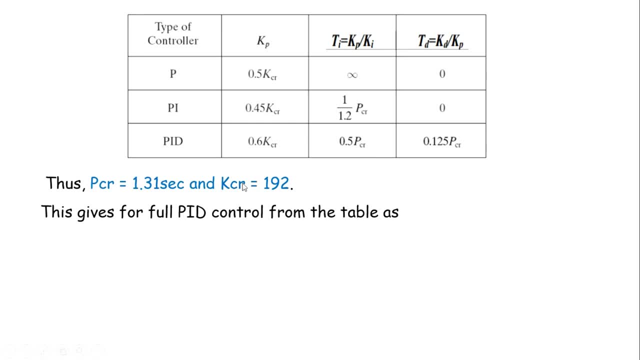 roots table, filler table, solar record table. we are going to find out the value of ti and td based on the value of pcr and kcr. now from the table you can find out the value of k, p i get. the value of kp is equal to 115.2, value of ki is equal to 175.87 and value of kd. 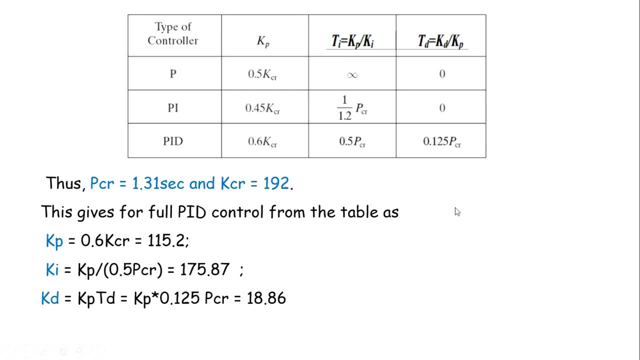 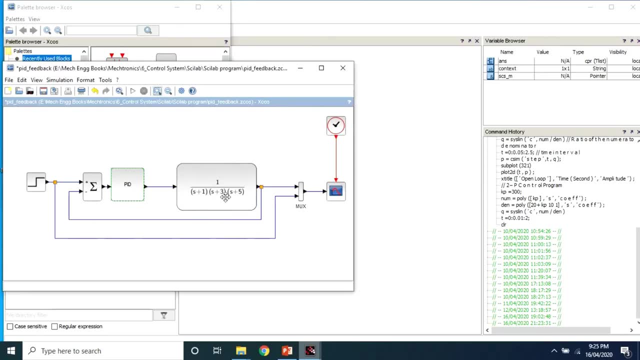 is equal to 18.86. go to that transfer function which i have developed in the psi lab excuse module. now, in that i am going to change the value of proportional integral and derivative controller as we already found this value now see the response curve. see this is the. 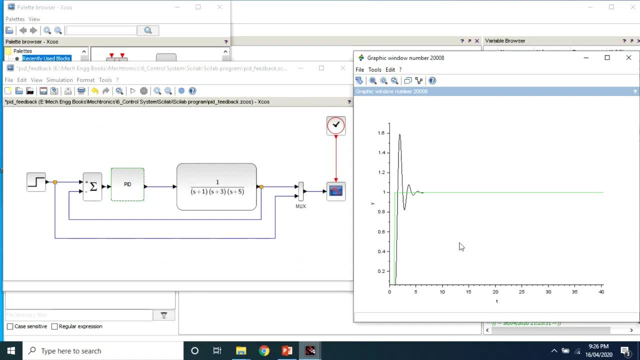 response curve for the given value of kp, ki and kd. here near about the 50 percent, we get the overshoot and if you look at here, steady state is, error is completely eliminated. rise time is also reduced. let us summarize the ziegler nichols tuning method: ziegler nichols. 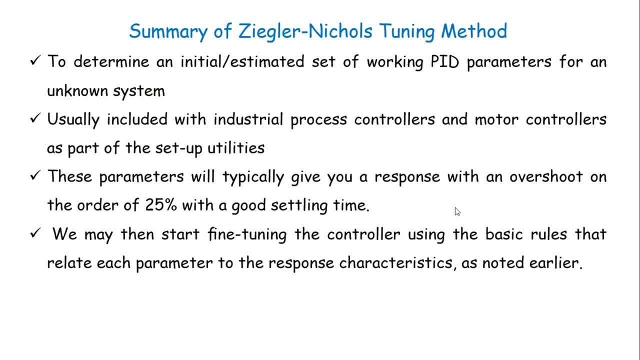 tuning method is used to determine an initial estimated set of working pid parameters for an unknown system usually includes the industrial process controllers and motor controllers as a part of the setup utilities. some controllers have additional attitudine routines. these parameters will typically give you a response with an overshoot on the order of 25. with a good settling time, we may then 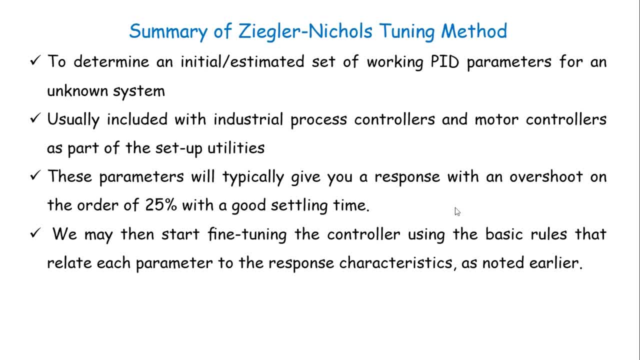 start fine tuning the controller using the basic rules that relate each parameter to the response characteristics, as noted earlier. thanks for watching this video. for more details, watch my other videos on the controllers.